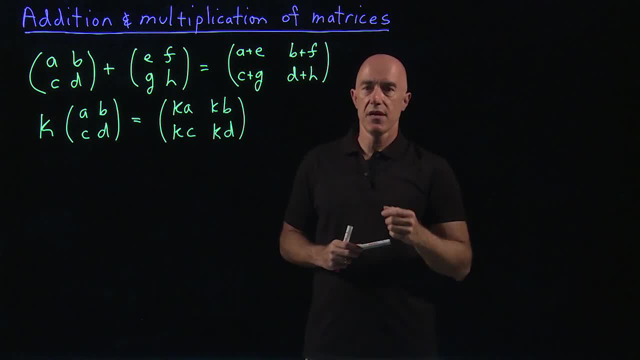 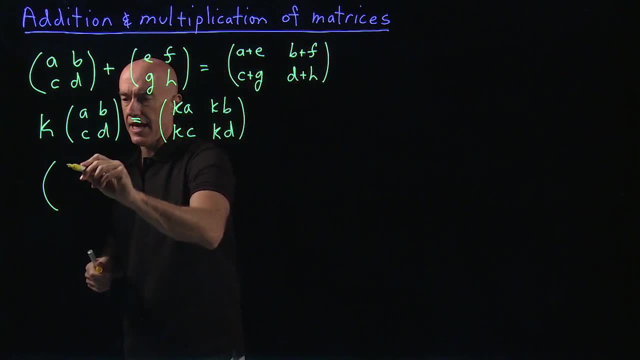 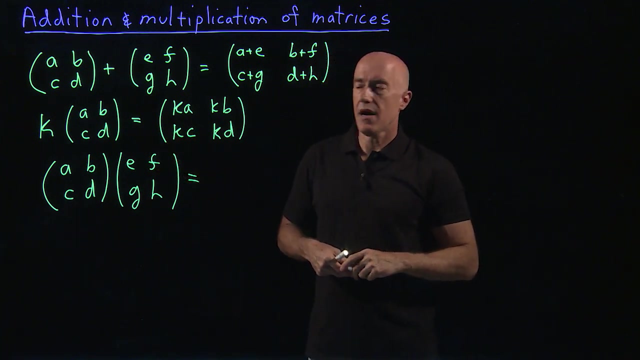 are actually multiplying two matrices. So let's multiply two two-by-two matrices. So here we have, say, A, B, C, D times E, F, G, H. So let's multiply two two-by-two matrices- G, H. So you might think that you can multiply each of the elements separately. The mathematical. 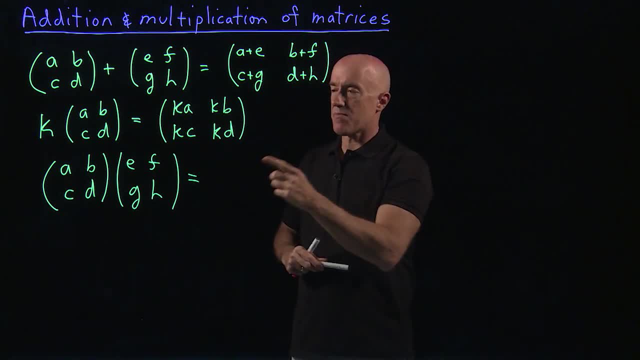 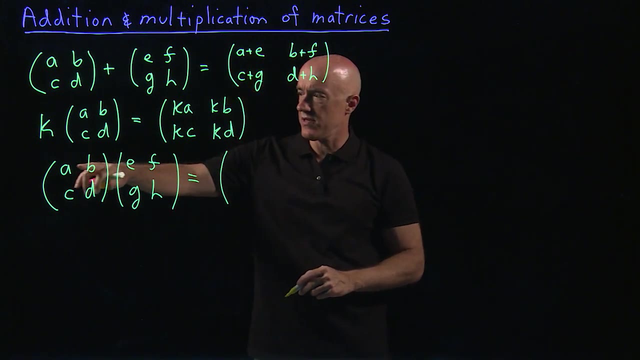 software called Matlab actually has an operation that lets you do that. But in general when you do matrix multiplication you have to do it very specially. And let me illustrate here with the two-by-two times two-by-two case: What you do is you go across the first. 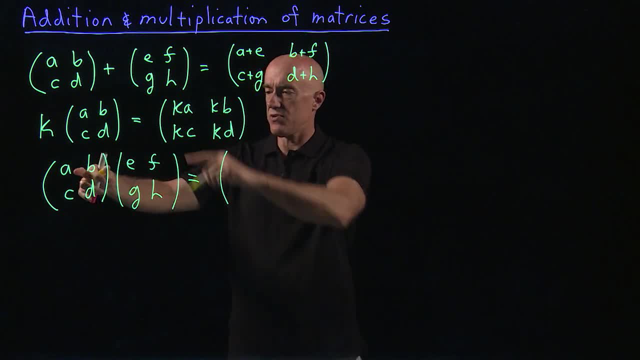 row. You go across the rows of the first matrix and down the columns of the second matrix. So here this first element would be across the first row of the first matrix, down the first column of the second matrix, So it would be A E plus B G, Then the element in the 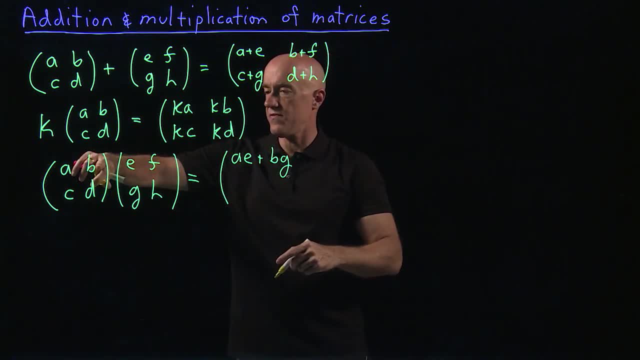 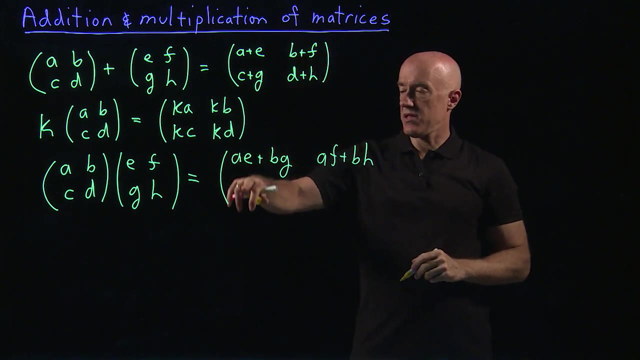 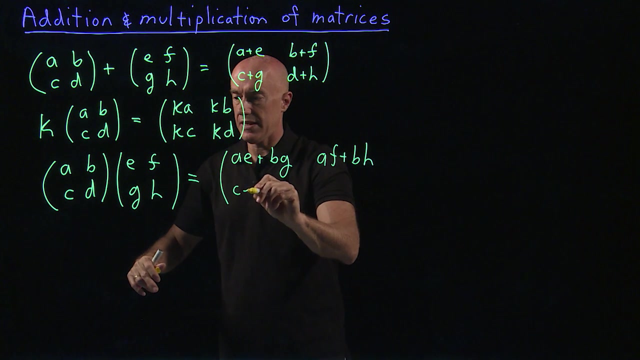 first row second column would be across the first row of the first matrix down the second column of the second matrix, So that would be A F plus B H. Then the element in the second row first column would be across the second row down the first column, So C, E. 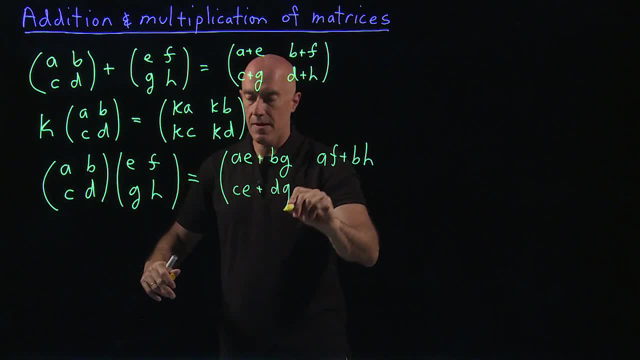 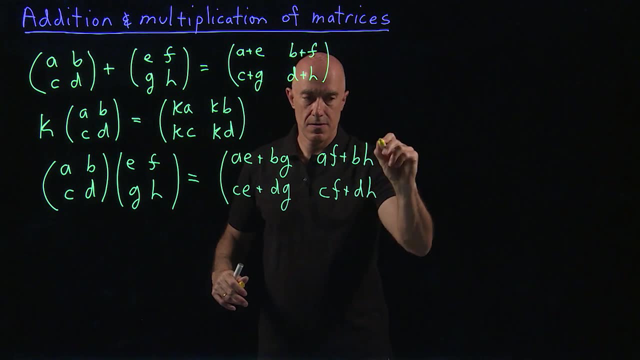 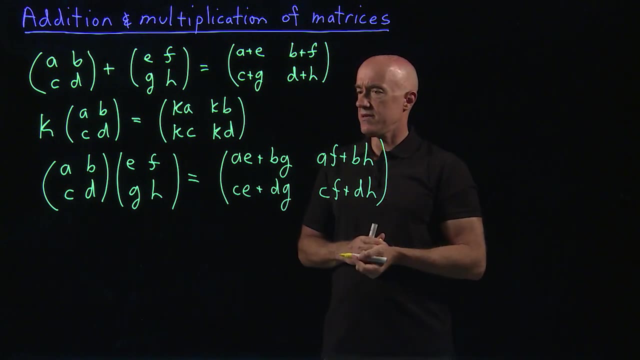 plus D, G And finally, the last element would be C, F plus D, H. So a matrix multiplication is a little bit tricky, but once you get the hang of it it's quite simple. An interesting thing about matrices that is actually very important is that they don't. 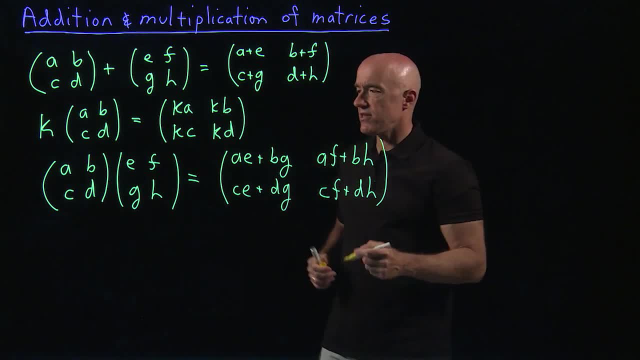 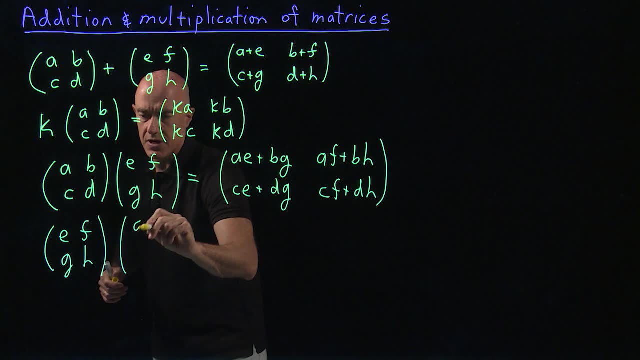 commute under multiplication. So if we change the order here- So let's say we did E, F, G, H, times A, B, C, D- If these matrices were numbers, you would get this particular number. So I've got C, B, C, D and so on. This is what we're trying to do here. So if these matrices 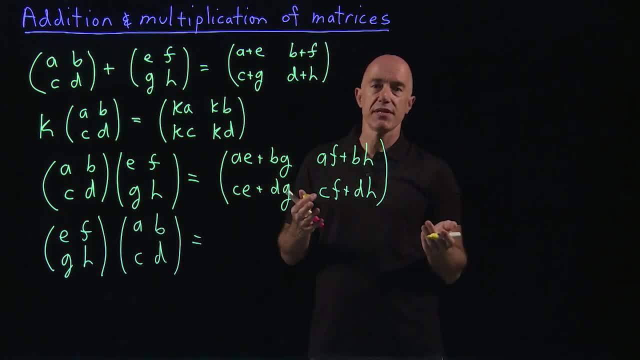 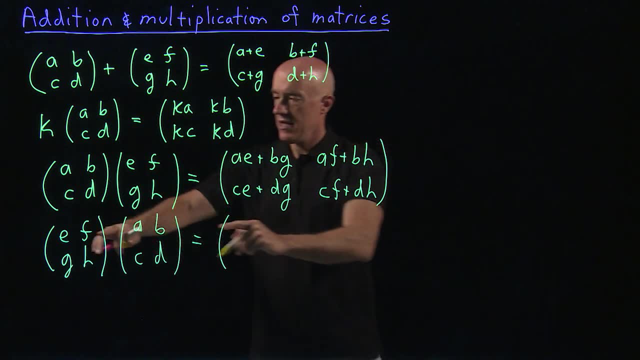 were numbers, you would get this particular number. But if they didn't, if they were a, the same result. but matrices are not numbers, so we have to follow the same rule of arithmetic here and let's see what we get here we have. so usually you write the element, the matrix, on the left, you 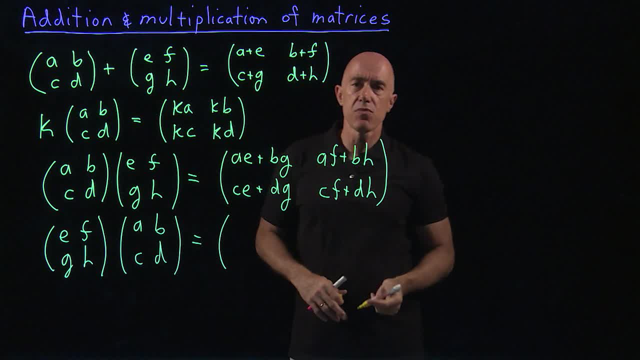 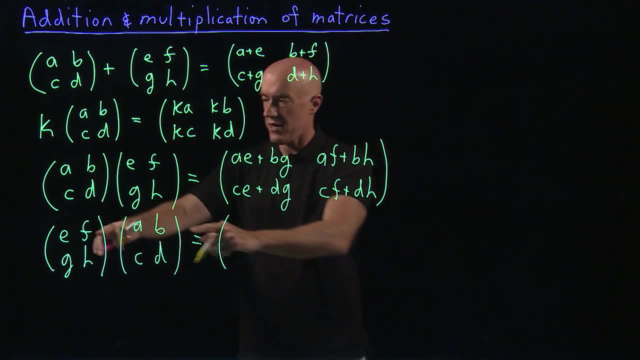 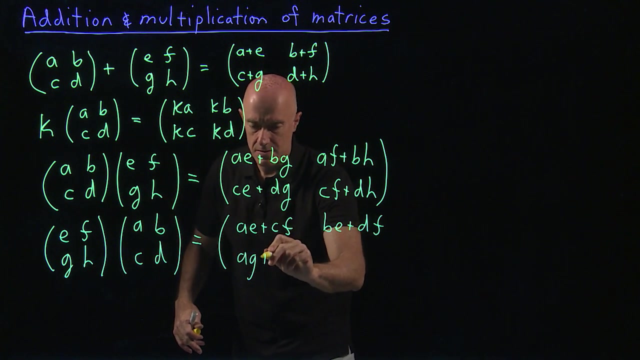 write the element on the left. but you know regular multiplication commutes. so just to be able to make a comparison, let me keep the alphabetical order here. so it would be AE plus CF and then it would be BE plus DF, and then second row, first column AG plus CH and then finally BG plus DH. 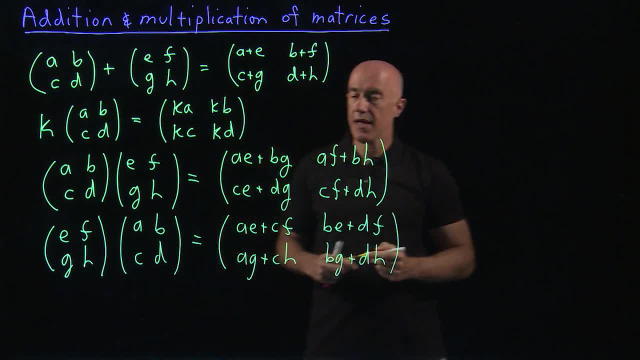 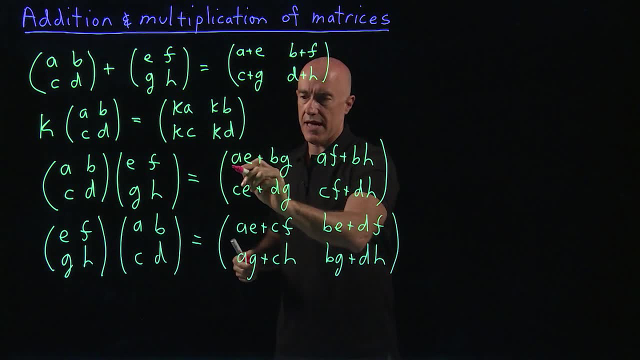 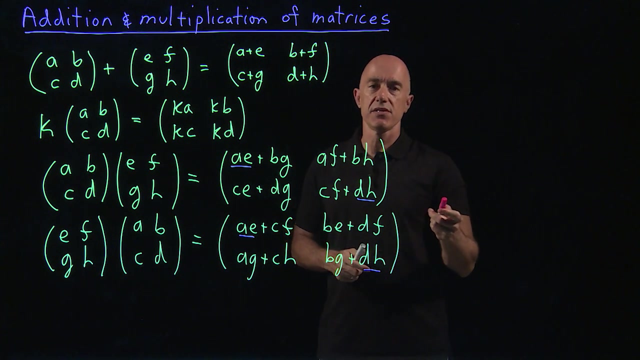 okay, we can look at these two matrices. are they the same? no, you get this. ones are the same and let's see here this is the same, but other than that, these are two very different matrices. okay, so matrices do not commute. that's very important to remember. 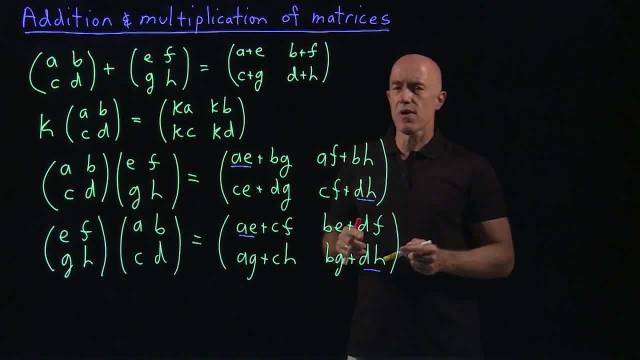 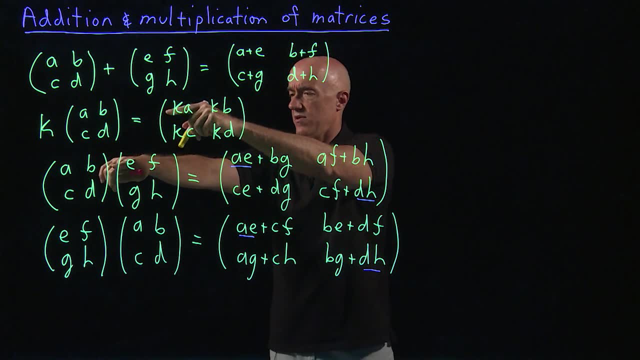 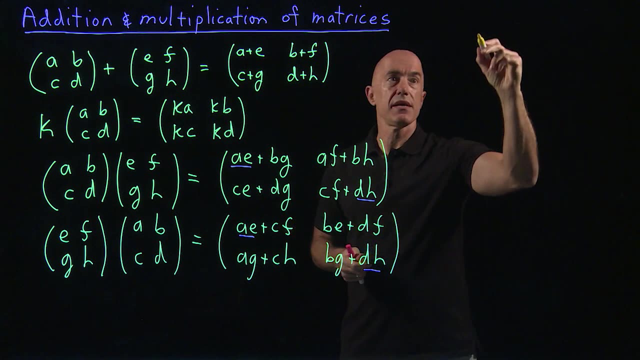 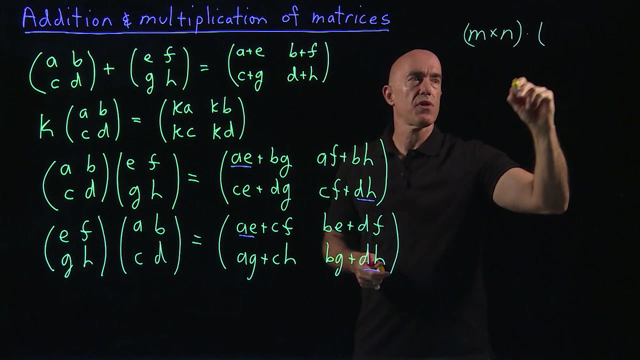 okay, so. So, as you saw, when we did matrix multiplication, we went across the columns of the first matrix and down the rows of the second matrix. So what does that mean? So the first matrix might be m by n, right. And then what size matrix can we multiply an m by n? matrix by: 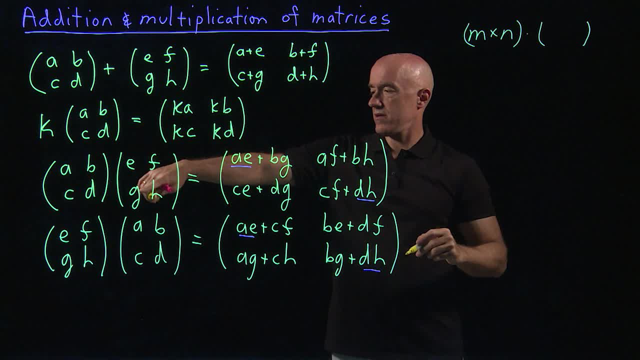 So we're going across the columns, right When you have the first row and then you go across the column. So that means we're going across the n columns. So we're fixing the row, going across the n columns and then going down the same number of rows. 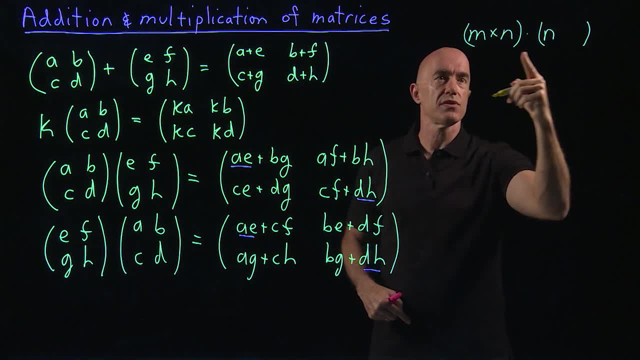 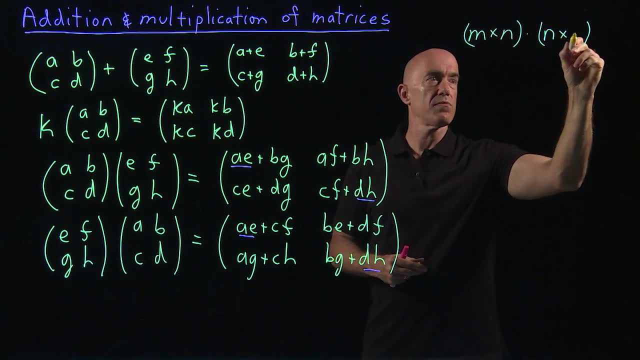 So the second matrix has to have the same number of rows as the first matrix has columns. So this is very important for matrix multiplication. And then the number of columns here is free. So the first matrix can have an arbitrary number of rows and the second matrix can have an arbitrary number of columns. 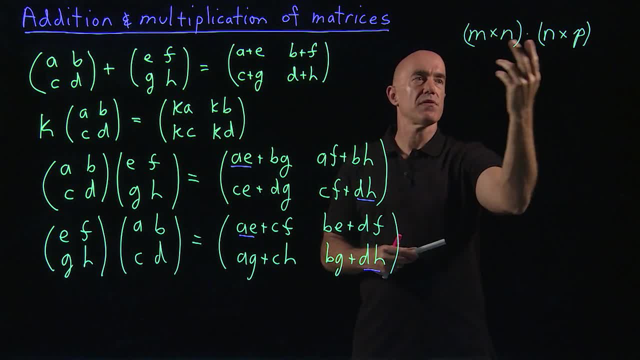 But the number of columns of the first matrix have to match the number of rows of the second matrix. Okay, it's a little bit tricky, But then if you do this properly, then you end up with a matrix which is m by p. 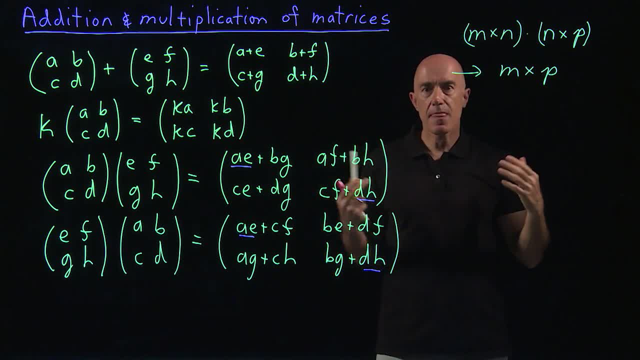 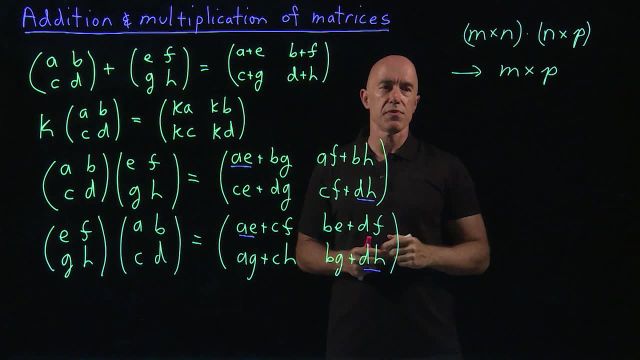 Right m by p. Okay, so for theoretical purposes it's useful to have a formula for matrix multiplication. So if we have two matrices, say we have c which is a product of two matrices, a and b, it would be nice to have a formula for the matrix elements of c. 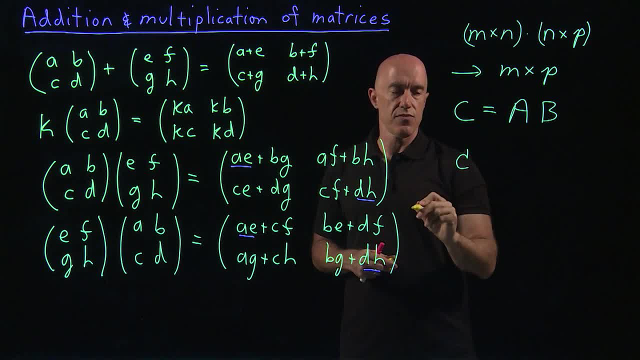 So what we do is we call them little c, right? And let's say we're looking at the element in the i-th row and the j-th column. So we're looking at c, i, j. How do we get the element in the i-th row and the j-th column? 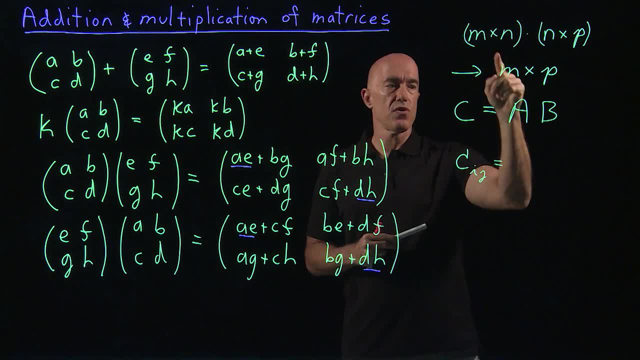 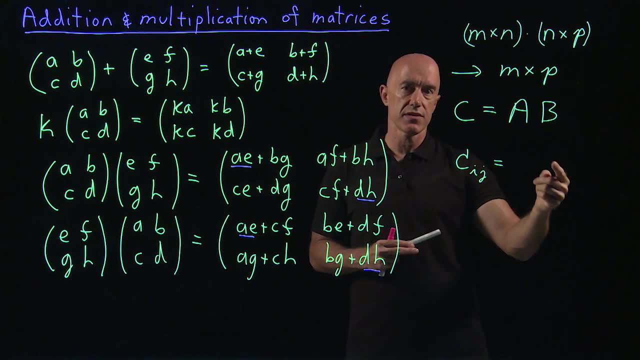 So we're going across the i-th row of the first matrix, which is the a matrix, and down the j-th column of the second matrix, which is the b matrix, and we're multiplying them, right? So I'm going to use this symbol. 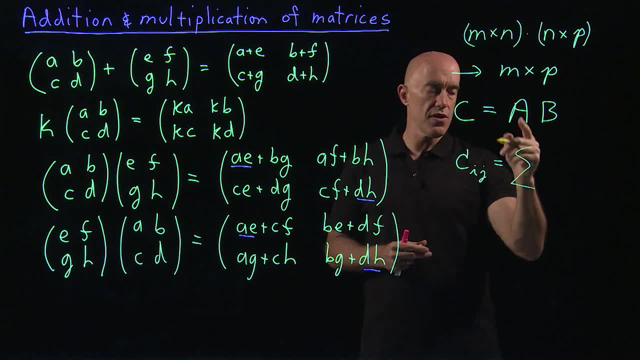 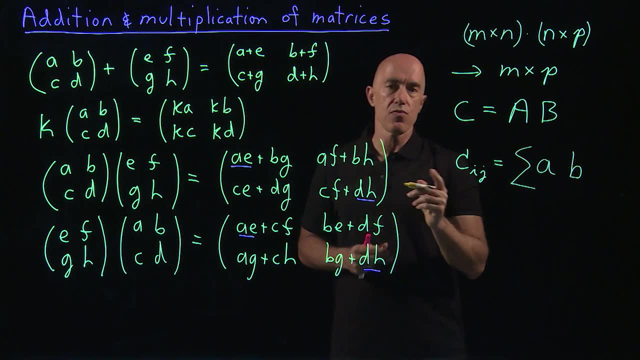 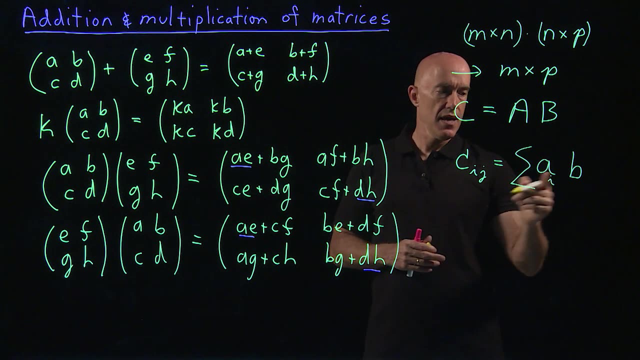 this symbol for summation. that means you sum. So the first element is a right, The second element is b. and where are we on the matrix right? The first one: we're going across the i-th row, so I put a subscript i. and the second matrix: we're going down the j-th column. 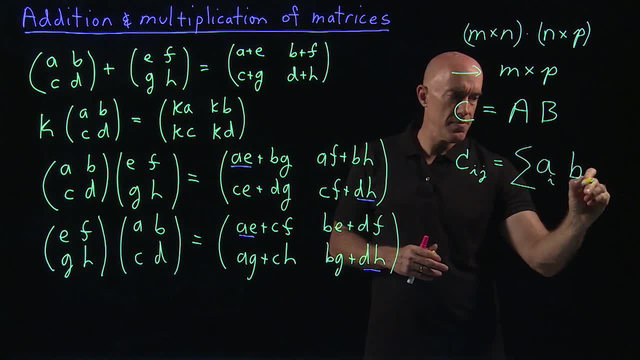 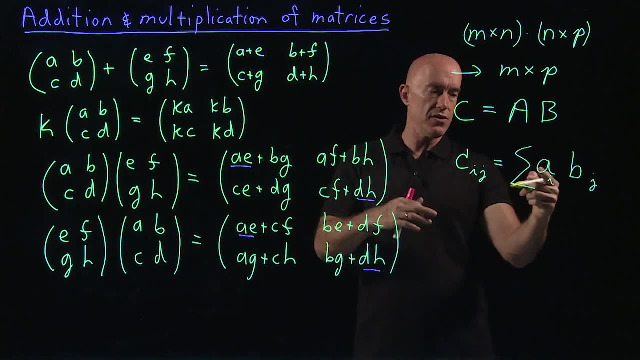 So the second index of b should be j, and then we're making a product of a, again b, as we go down the i-th row, as we go across- sorry, across the i-th row and down the j-th column. 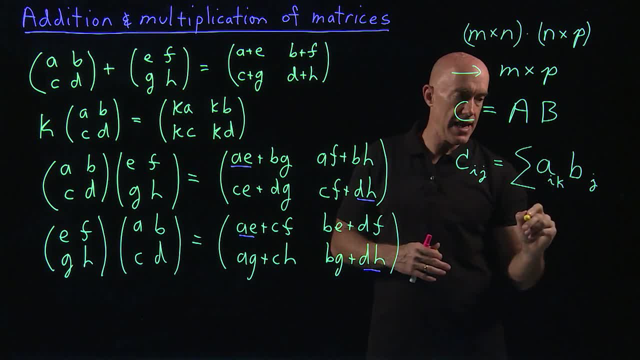 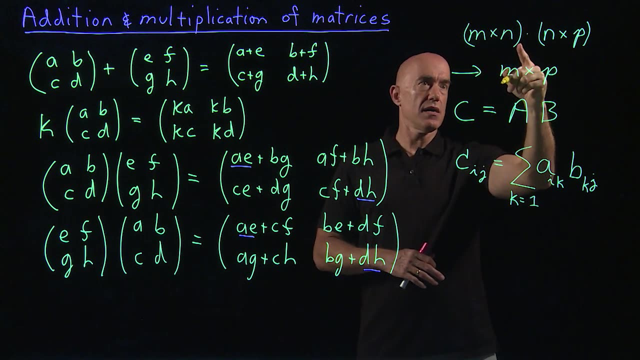 So this second index- here I can say k, and this first index, here I can say k. and then we're summing from k equals 1 up to how many we have here. So this is supposed to be m by n times n by p, so we have n.